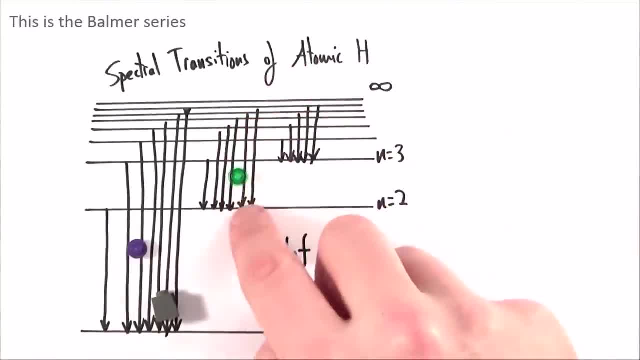 frequency isn't as big and therefore we maybe have visible light given off at this part of the spectrum. And finally, these are fairly small energy changes over here, so we might have infrared light or infrared photons which are given off, And effectively you can only have certain values of photons given off and therefore certain values of wavelength of light which are emitted by hydrogen. 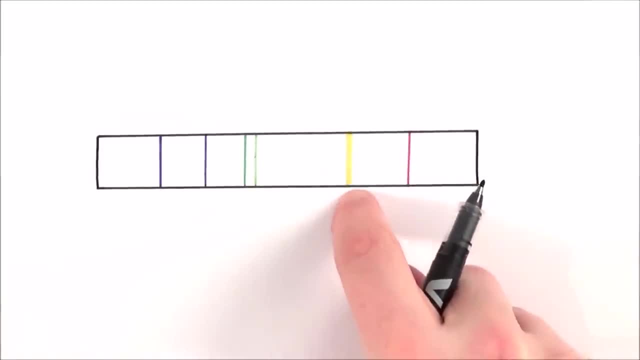 What we can actually do is look at the various colors of these emitted photons, And what I have here isn't actually hydrogen. this is helium, And what we can look at are the various wavelengths of light which are emitted And effectively, we have the visible. 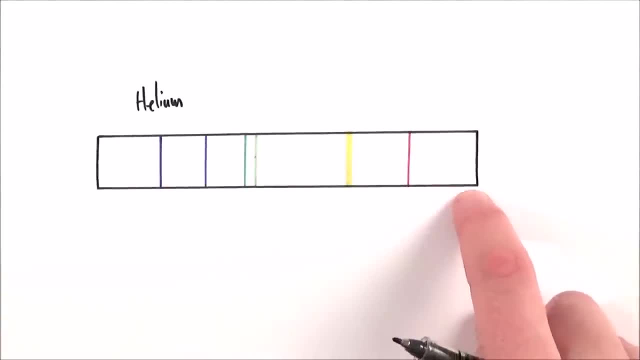 spectrum here going from the violet end right through to the red, And what we call this is an emission spectrum. This emission spectra shows a certain wavelength of photons which are given off by helium. As it's excited, we might have a lot of helium gas, which is really hot and full of lots of. 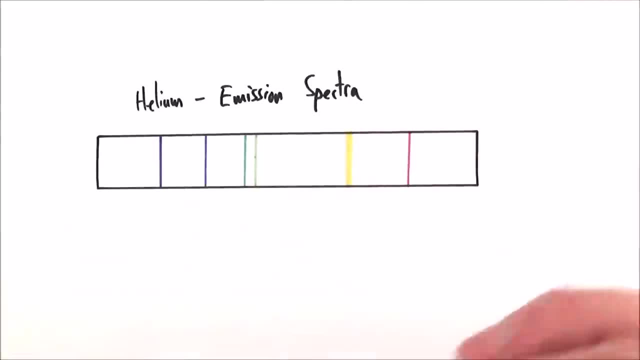 energy, and as the electrons drop back down to the various ground states and the lower energy levels, they emit certain wavelengths of light, And for every single element it has its own particular emission spectra. How do we see this? Well, we see all the colours mixed together, so we might see the yellow adding to the red. 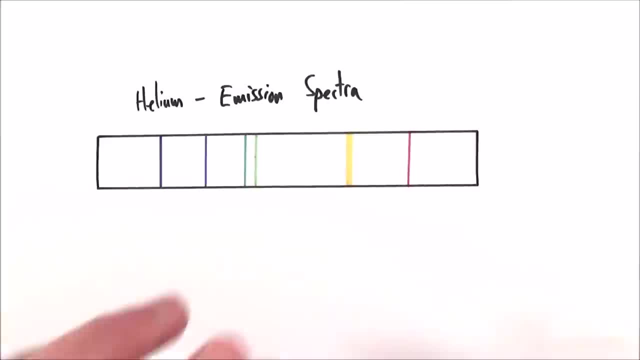 to the green, to the blue and the violet, and what we might see is white light. So how do we actually get this spectra? What we have to do is we need to shine that white light through a diffraction grating, and what this does is it splits up that rainbow of colour and really shows us the certain 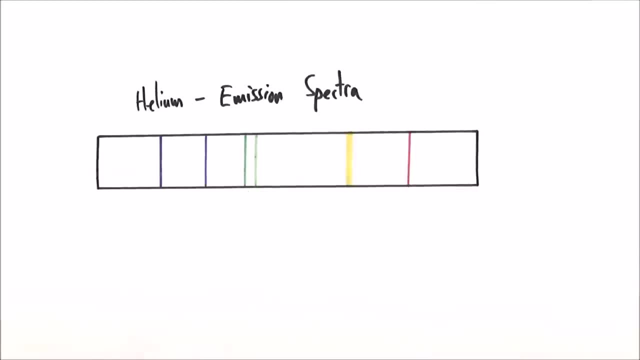 frequencies of light that make it up. However, this emission spectra also has its kind of twin brother, and this isn't so much things being emitted, but this is things being absorbed. Now we've already seen on the model that when an electron drops down, it emits a certain 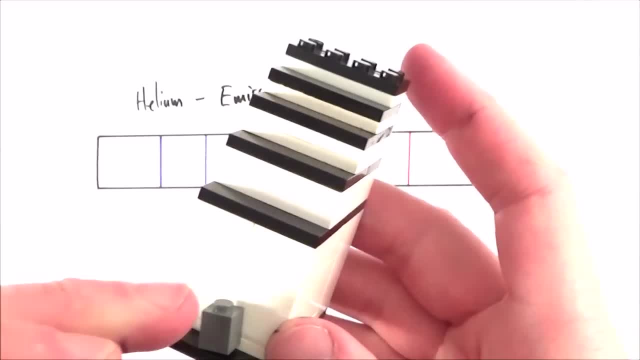 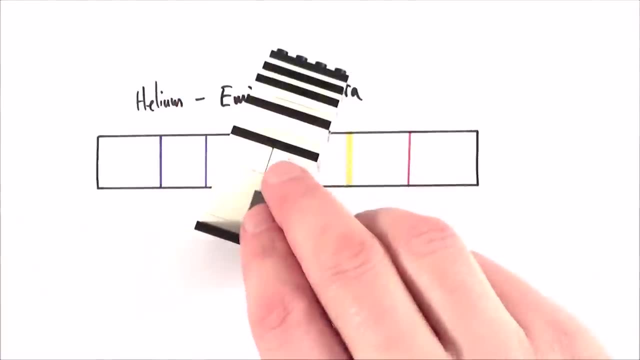 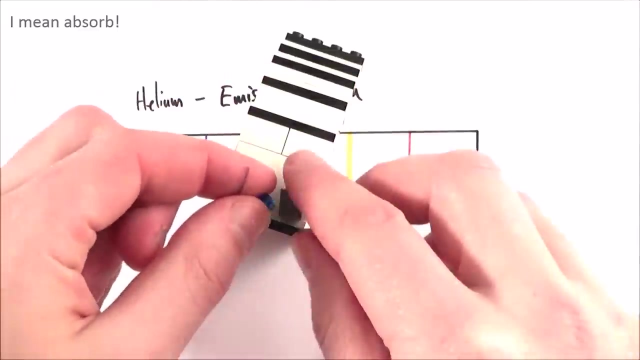 photon of a certain frequency. Well, in actual fact, when this goes up to the next wavelength, It only emits or only absorbs certain frequencies of radiation. So this one here, maybe, might emit a photon with a blue wavelength which goes out, But in order for it to get up to the next level it has to emit a blue photon. 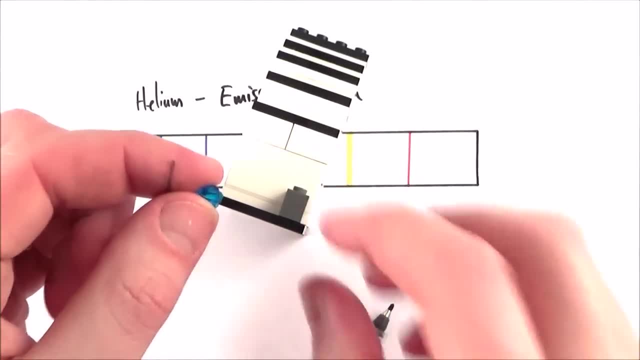 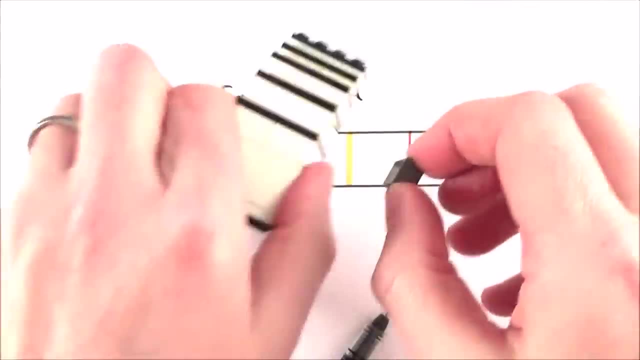 A red photon, a green photon, these don't have quite the right energy. It's very, very picky about who it chooses. So this photon comes in, it excites the electron and it moves up an energy level And therefore what we have is not just an emission spectra, but we also can see an absorption. 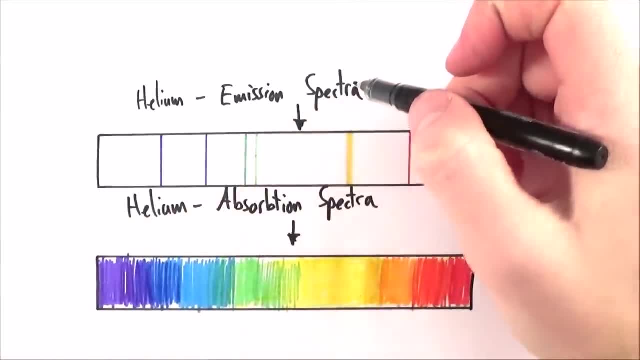 spectra, An emission spectra, An emission spectra, An emission spectra is something, but an absorption spectra is when you maybe have a cool gas and you shine a load of white light through it, So white light being made up of all of the colours of the rainbow. 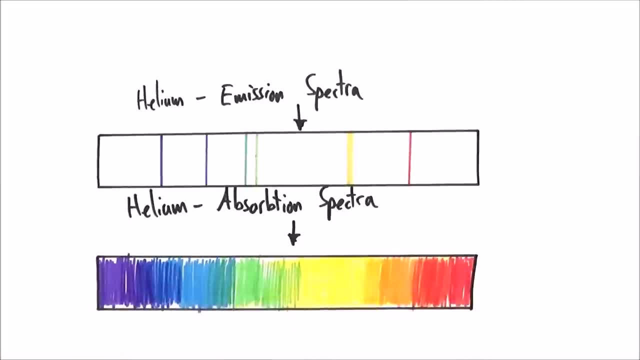 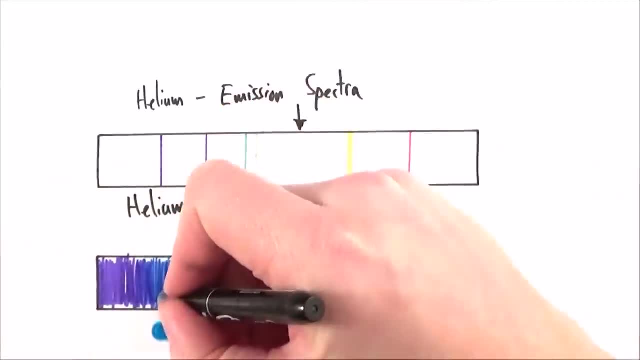 And what we find is that only certain colours or only certain photons are actually absorbed by whatever we've got, And what we see is kind of, I guess, like an anti-emission spectrum, And we see a black line where no light kind of gets through. 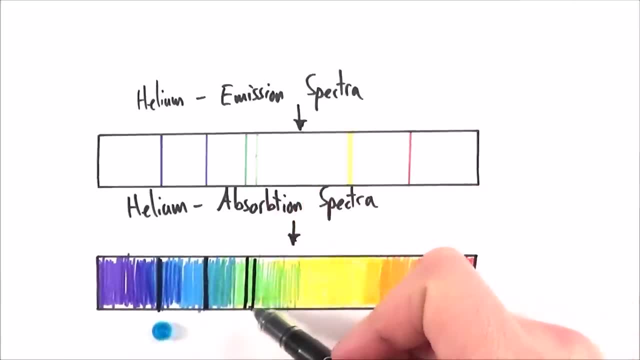 So we find that actually, certain frequencies of green light are absorbed And therefore there's like a basically a bit of a gap in the spectra, And this is really, really important. okay, This gives us evidence for the fact that what's inside stars, that there is actually helium. 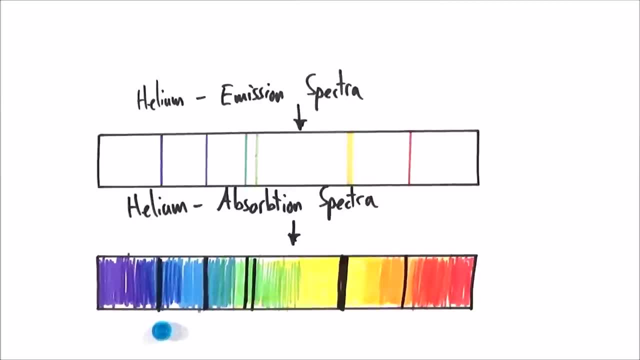 inside stars. It gives us evidence for the fact that the galaxy and the universe in fact- well, not the galaxy, but the whole universe- is expanding, And it's because what we can do is by looking at star light. we can start to see the various 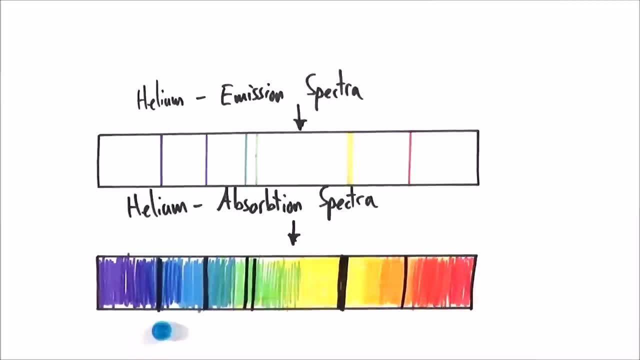 chemical elements that make up the kind of the outer atmosphere of those stars. So an absorption spectra is where certain frequencies of light are missing because they're being absorbed by that element. So we know that helium absorbs certain yellow, red and green and sort of different frequencies. 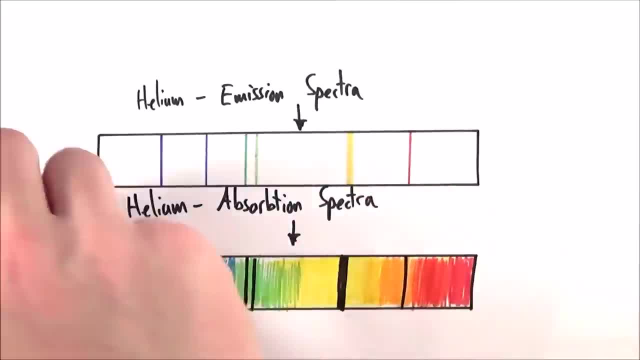 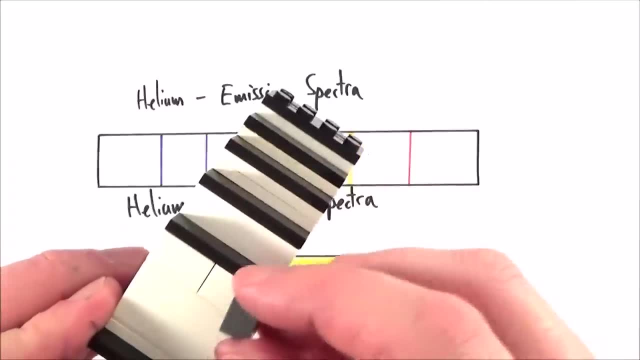 like that, Whereas when it emits stuff it only emits the same things, And this is because the frequencies which are absorbed by the electrons to move up the levels are the same as the photons given out when these things drop back down to their ground state. 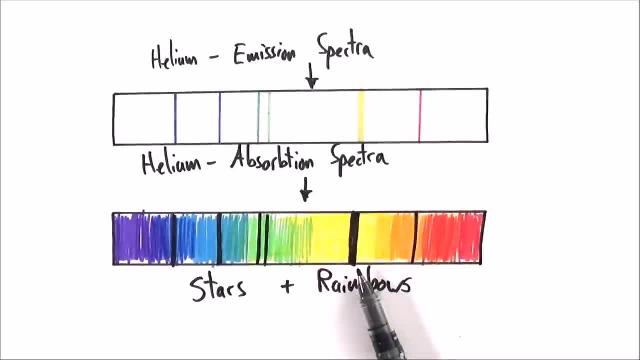 So that's what quantum physics really leads on: to Basically work on stars and rainbows And how, by knowing about what's inside the atom on a very, very smaller scale, We can then start to investigate things on the very largest scale in our universe.